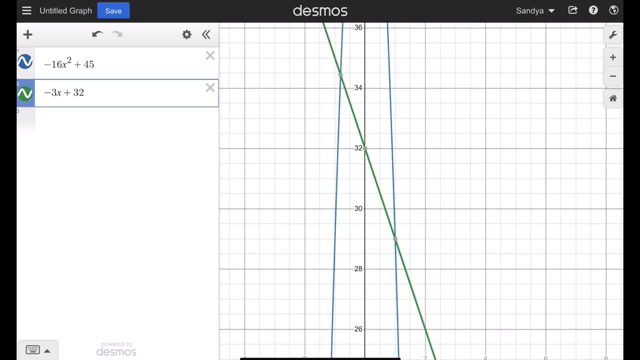 look for the intersection points to determine the solutions to my system. So this first point is negative: 0.81334.438.. And the second point is 1.29.. So let's think about these two solutions. So we know that our 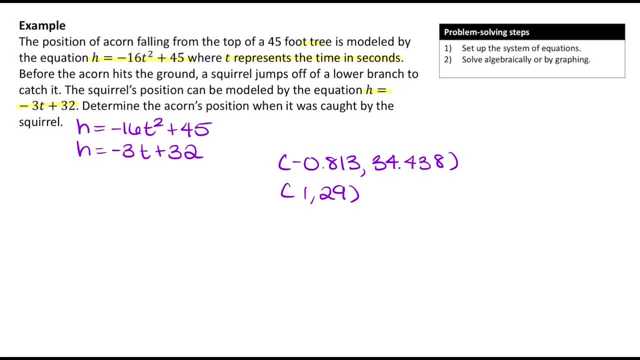 x-coordinate represents t and in this case t represents time. So here you can see: we have a negative value for t. so this solution is actually not going to make sense in the context of our problem, because we cannot have negative values for time. Well, the second solution, that's telling. 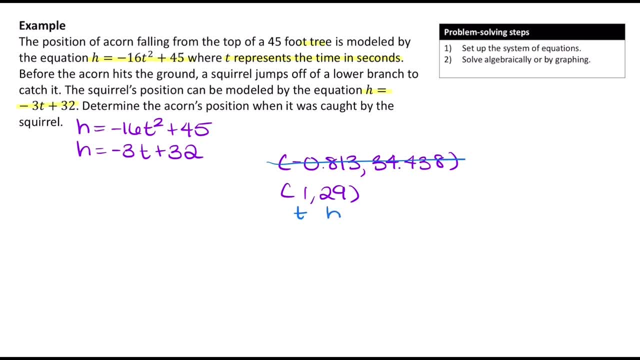 us that time equals one second and the height is going to equal 29.. Those are both reasonable values so we can use that solution. So we'll say that the unicorn's position will be 29 feet above ground and we know that that's going to happen one second. 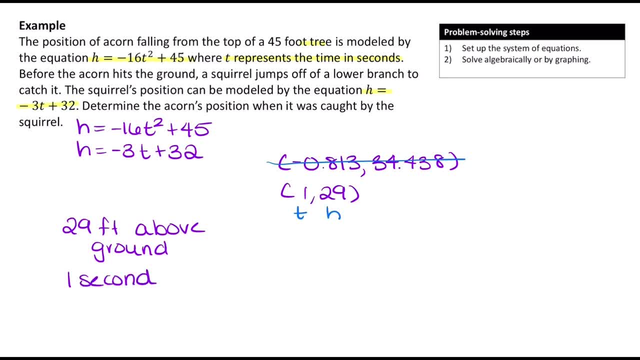 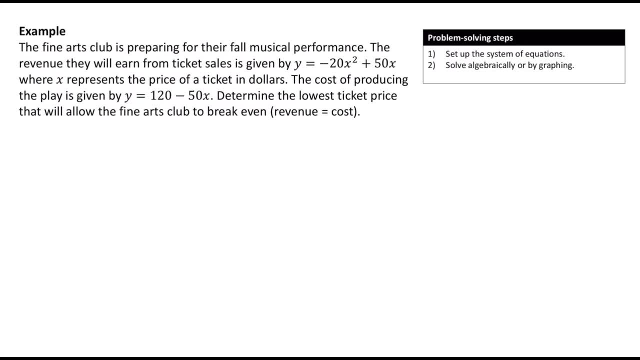 after it begins to fall. So now let's try this example. It says that the Fine Arts Club is preparing for their fall musical performance. The revenue they will earn from ticket sales is given by y equals negative 20x squared plus 50x, where x represents the price of a ticket in dollars. 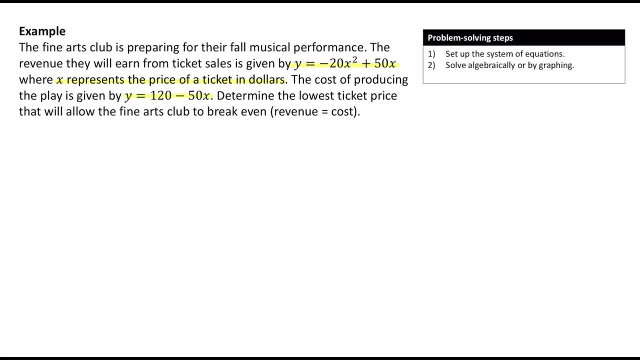 The cost of producing the play is given by y equals 120 minus 50x. Determine the lowest ticket price that will allow the Fine Arts Club to break even where their revenue equals their cost. So we know that we want revenue to equal cost. so revenue is given by negative 20x squared plus 50x and the cost is given by 120 minus 50x. 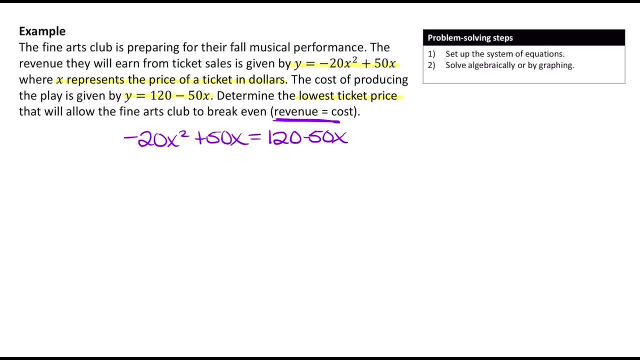 So this is a quadratic equation, so I know that to solve this I need to set it equal to zero, and I can do that by subtracting 120 and adding 50x to both sides. So when I do that, that's going to now become the equation negative 20x squared. 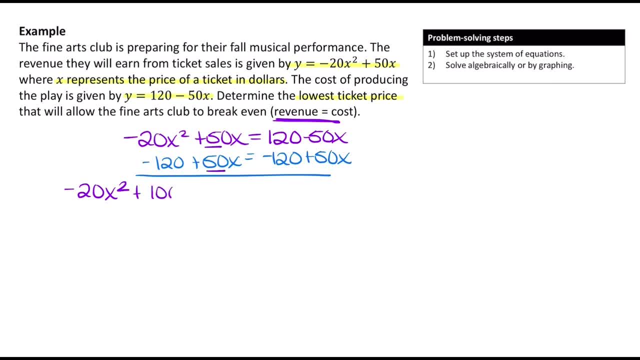 and then I have 50x plus 50x, which is plus 100x, and then minus 120 equals zero. Well, notice that all of these terms have a GCF. The GCF of all these terms is negative 20,. 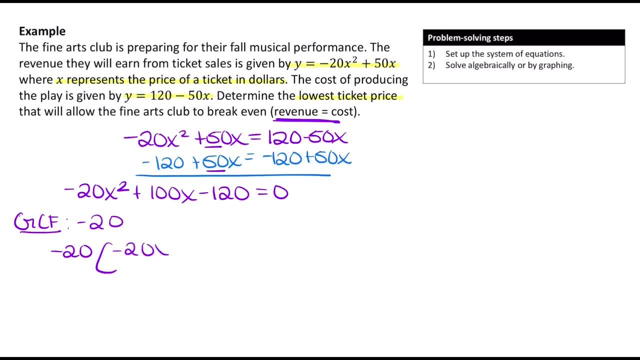 so I can go ahead and divide everything by negative 20.. So I have negative 20x squared divided by negative 20,, plus 100x divided by negative 20, and then minus 120 equals zero. So I have negative 20 times negative 20 over negative 20 cancels. so I have x squared. 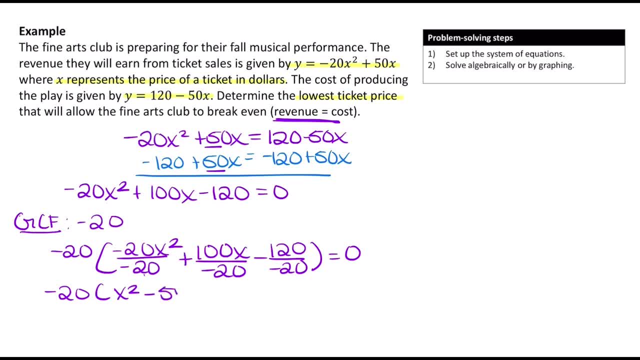 and then plus 100 over negative 20,, that's going to be minus 5x, and then minus 120 over negative 20,, that's going to be plus 6, and that's equal to zero. So now to solve this, I can go ahead. 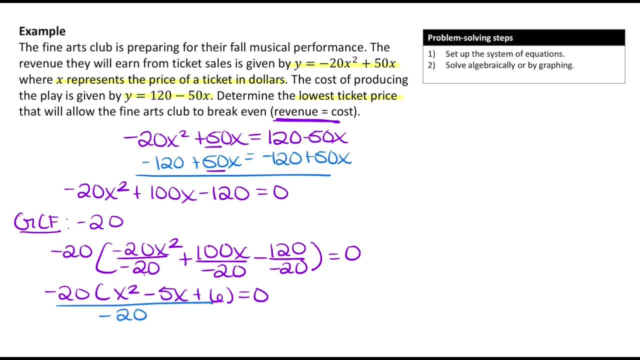 and divide both sides by negative 20.. So when I do that, I end up getting x squared over negative 20, squared minus 5x plus 6 equals zero. So I'm going to solve this by factoring. I need factors. 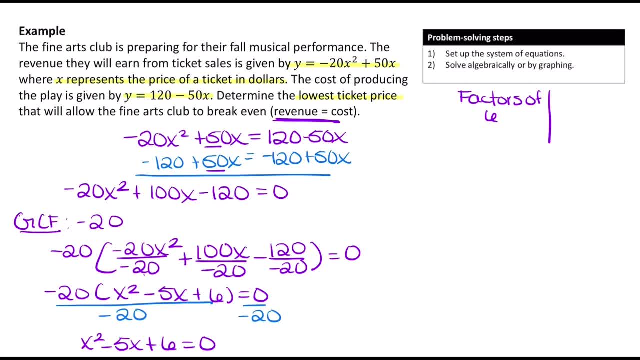 of 6 that are going to add to negative 5.. Okay so 6 is positive and 5 is negative. So I'm going to make two negative factors. So I have 1 and 6, and 2 and 3.. Okay so, negative 1 and negative 6. 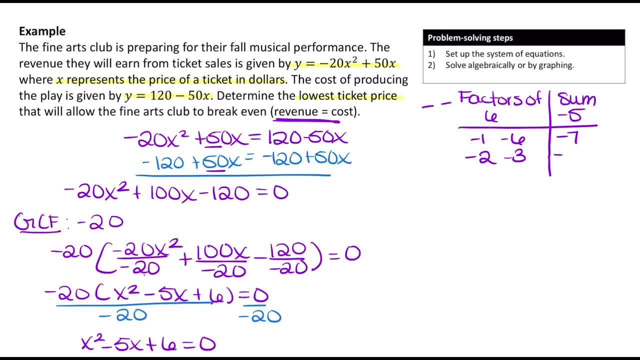 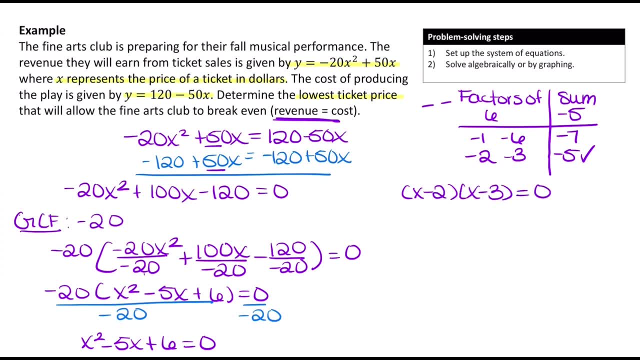 is negative 7, so that won't work. Negative 2 and negative 3 is negative 5, so that's correct pair. So I have x minus 2 times x minus 3 is zero. So I'm going to set each equation equal. 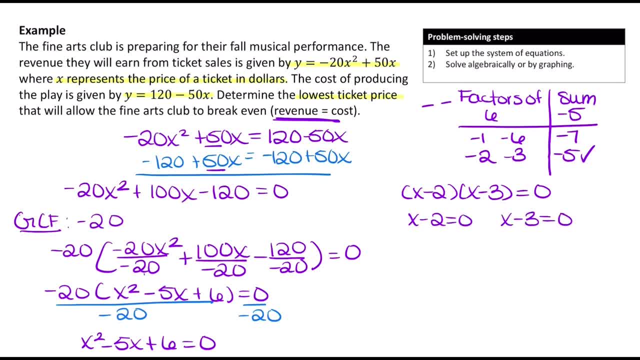 to zero and solve for x. So when I do that, here I'm going to add 2 to both sides, And so that's going to give me x equals 2.. And then over here I'm going to add 3 to both sides, which gives me: 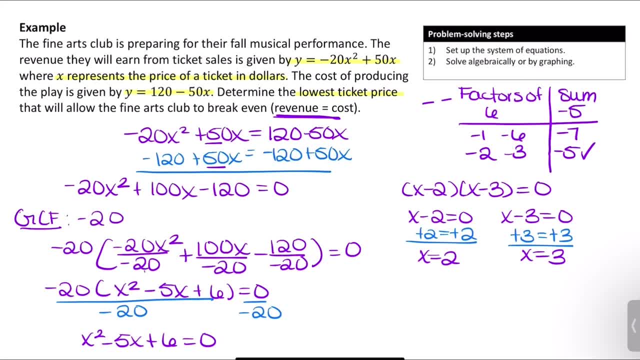 x equals 3.. Okay, so let's think about what this problem is asking us now. It's asking us to find the lowest ticket price that allows them to break even. Well, ticket price is x, so all it really is asking us for in this problem is the value of x. So we have two values of x: x equals 2 and x equals. 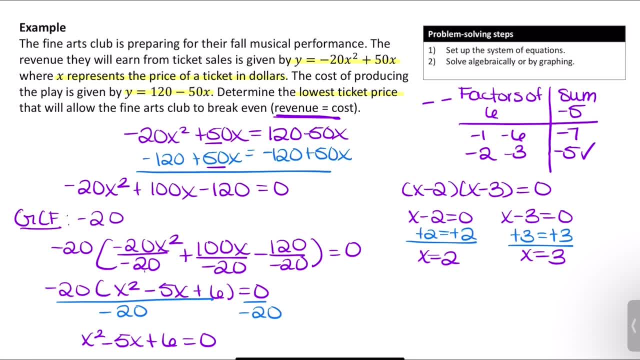 3,. that are both reasonable solutions, But the lowest price out of these two is going to be 2, so we're going to recommend that they charge $2 per ticket so that they can keep their prices low but then also break even. So now you can go ahead and pause the video and try doing this example on.